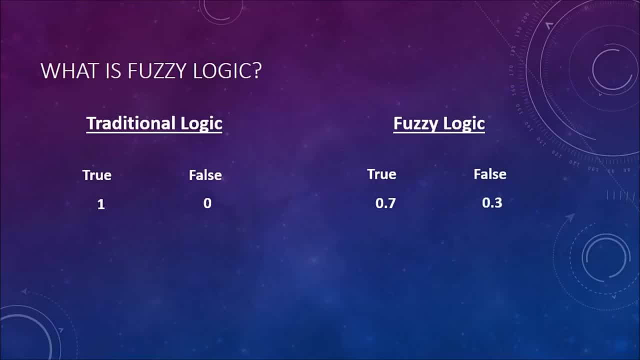 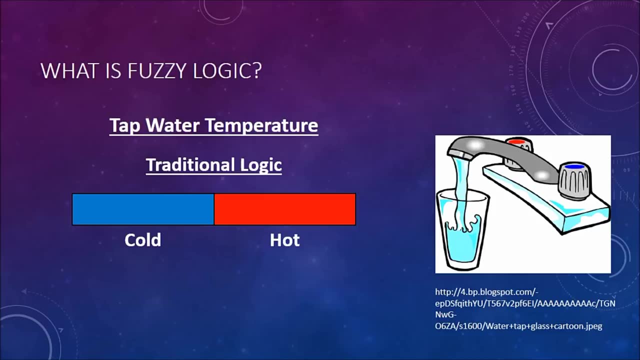 but only partially true with 0.7, or false. it's mostly false with 0.3.. So let's use tap water temperature as an example. In traditional logic, you would have this represented by either being hot or cold, representing 0 or 1 respectively. With fuzzy logic, you could have something like: 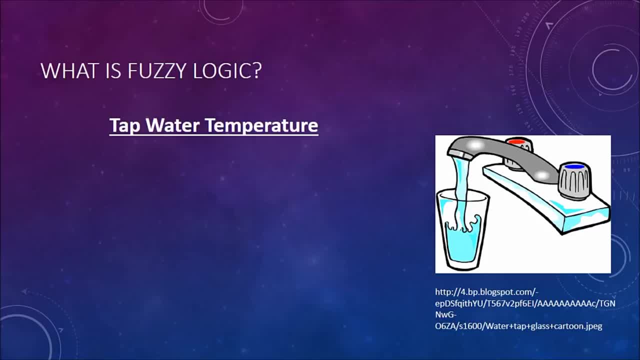 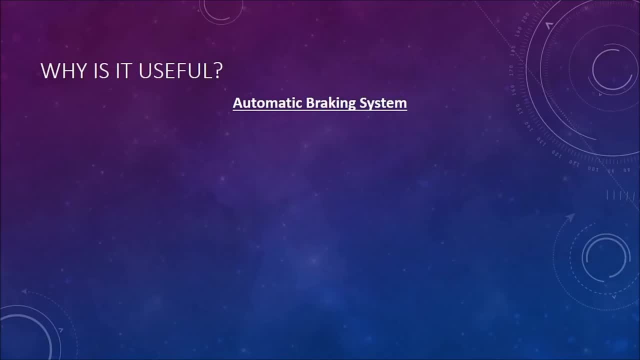 this, where you have a gradient from hot to cold, So you could have something that is lukewarm, very hot, slightly cold, etc. instead of just hot or cold. So why is it useful? Well, consider, you have an automatic braking system in your car that can decide when to brake, Using 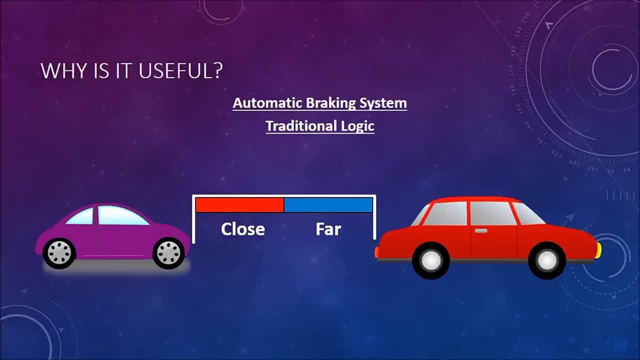 traditional logic, it might look something like this: where you have a car and you're driving a car in front of you that's far away or close and there's some value in between, where it switches, The car being close can either be yes or no, 0 or 1, and the brakes can either be on or 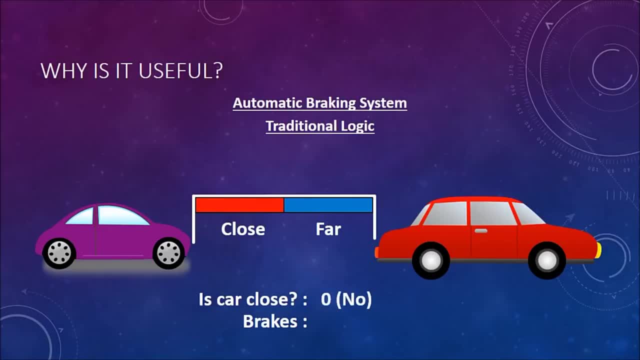 off, again, 0 or 1.. So, in this situation, the car is far away, so it's not close, and the brakes are off as a result of this. Now, in this situation, the car is now close, represented by 1, and the 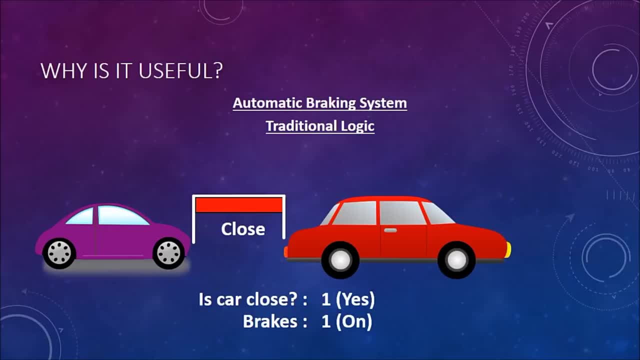 brakes are now represented by 1 as on. Now this might be a problem, because the car has now applied the brakes with full pressure and you're going to slow down very quickly. So you're going to slow down very quickly and you're going to slow down very quickly and you're going to slow down very. 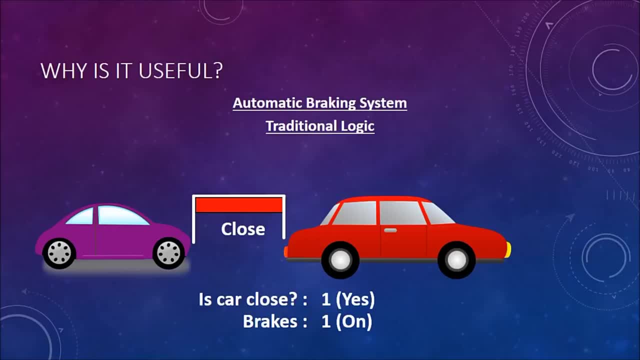 quickly, even though the car in front of you might not be approaching you very quickly. it might not be moving at all, And this puts huge stresses on the car, including the components like the suspension, the frame, not to mention the occupants. So, instead of doing something like 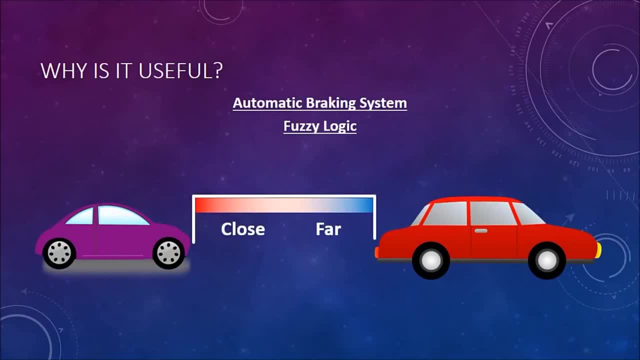 that. let's consider using fuzzy logic. So this is your situation and now, going from close to far, you have this gradient And you can say: is the car close? Well, it's anywhere between 0 and 1, this range, And the same thing with the brakes: you can apply pressure between 0 and 1.. So in 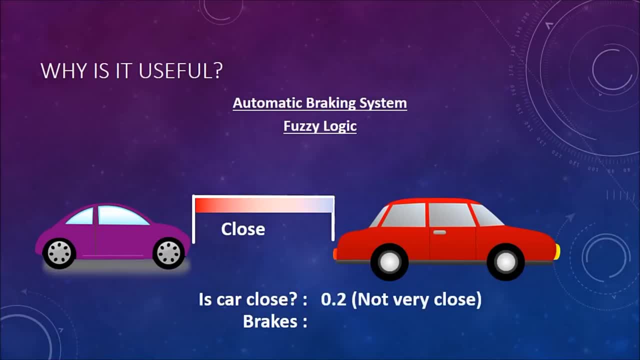 this situation is the car close? Well, 0.2.. It's not very close And, as a result, the brakes we're only going to put slight pressure on. And in this situation is the car close? 0.8,. 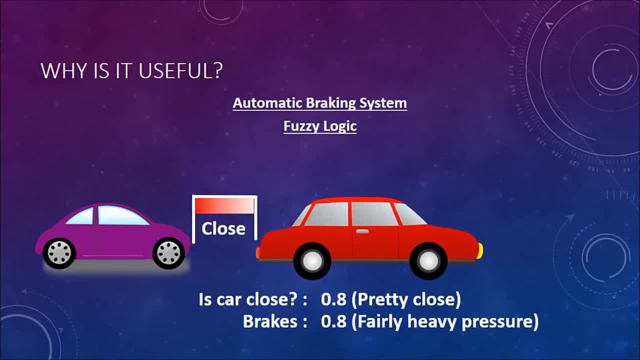 it's pretty close And, as a result, the brakes we're going to apply fairly heavy pressure to, and this will slow us more quickly. The result of this is that you get a much smoother output, depending on where the car is, and it's not just on or off for your brakes. This will put less